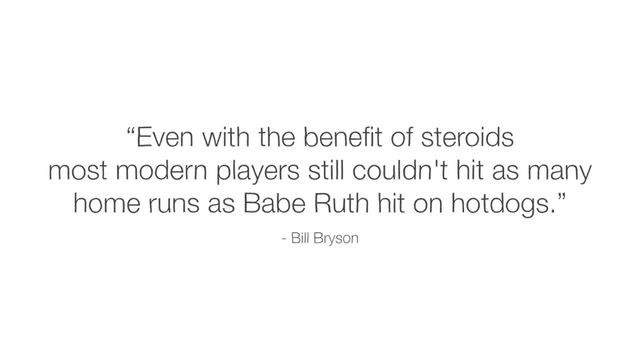 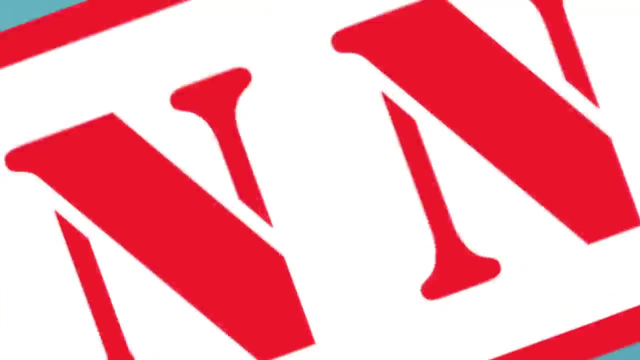 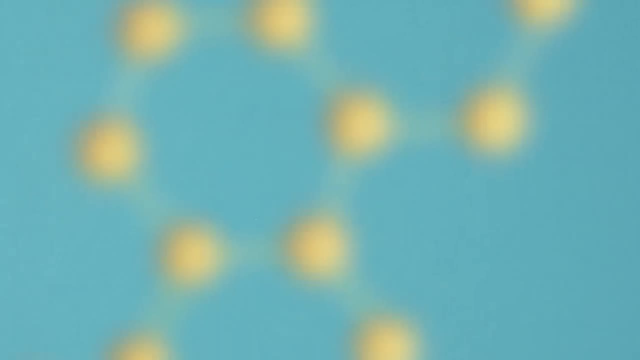 They've caused global scandals. They're banned in most athletic competitions. But are steroids actually bad for you? The term steroids refers to a broad category of molecules that share a similar molecular structure but have many different functions. When people talk about steroids in the context of sports, they're referring to a subset of steroids that resemble 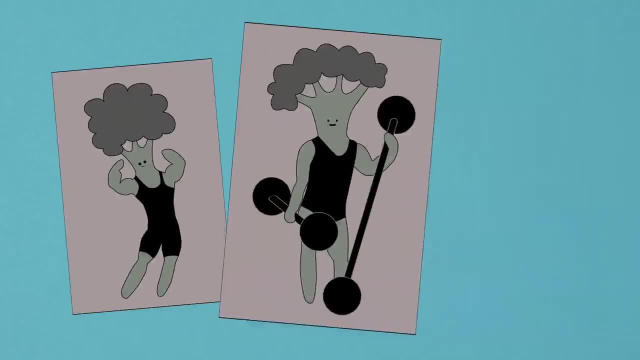 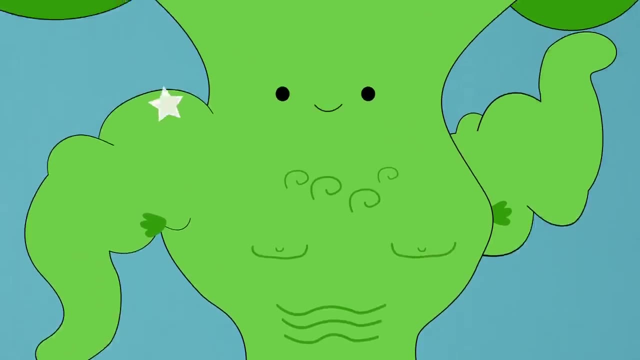 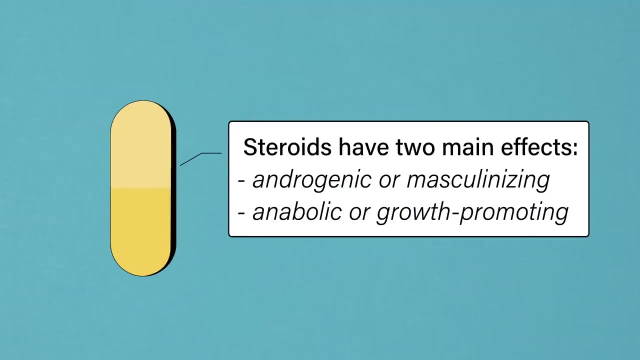 testosterone. Though elite athletes and bodybuilders began using these steroids in the 1950s, today most steroid users are actually not competitive athletes, but people seeking a particular appearance. These steroids have two main effects: androgenic or masculinizing. 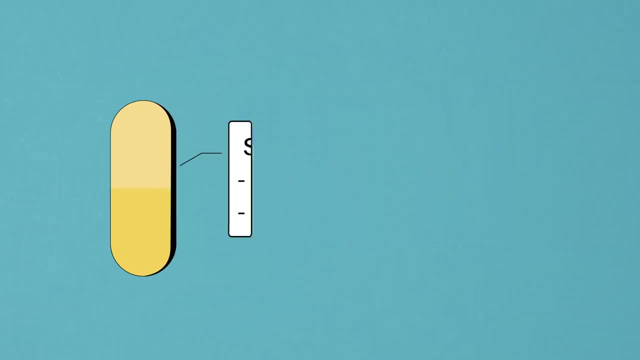 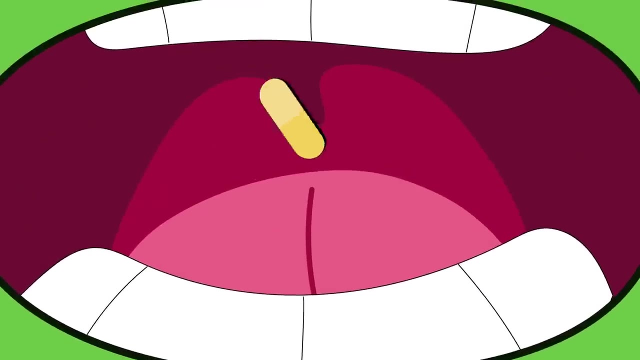 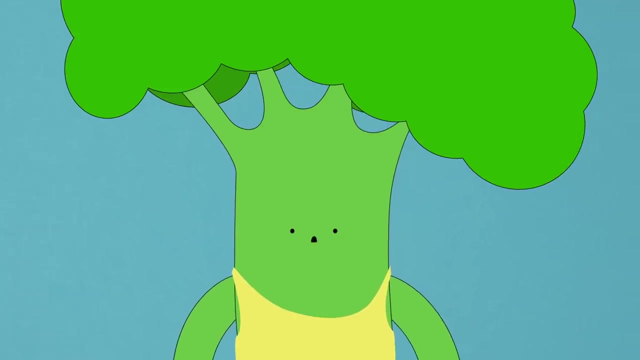 and anabolic or growth-promoting. These effects mimic naturally occurring testosterone, which drives the development and maintenance of male secondary sex characteristics and general growth in everyone. That means testosterone and the synthetic steroids based on it promote body and facial hair growth, enlargement of the vocal cords and deepening of the voice, increased muscle mass and strength. 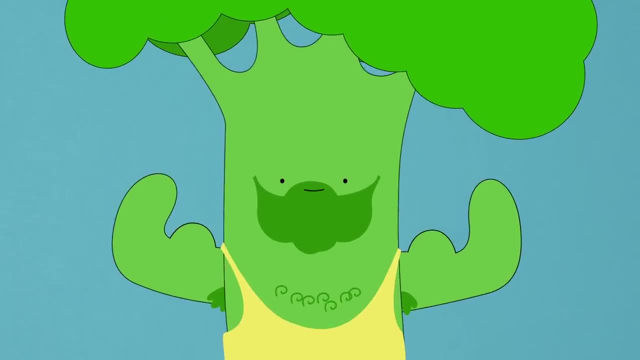 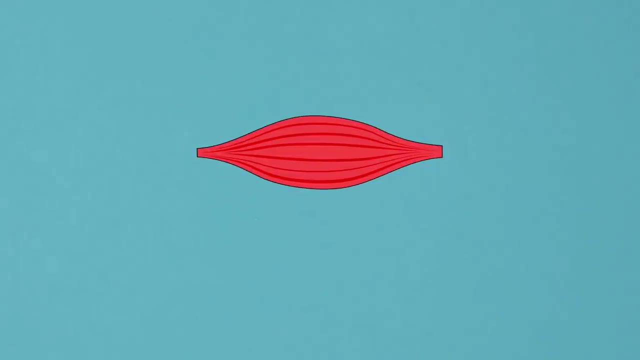 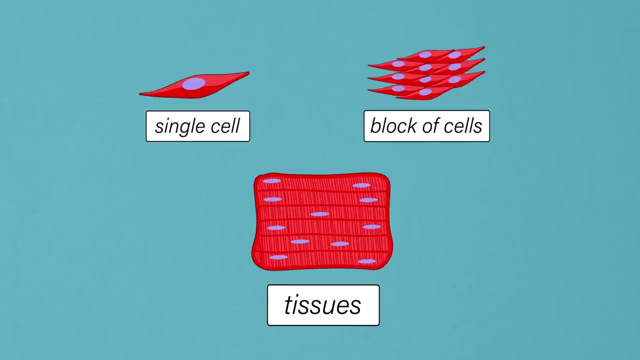 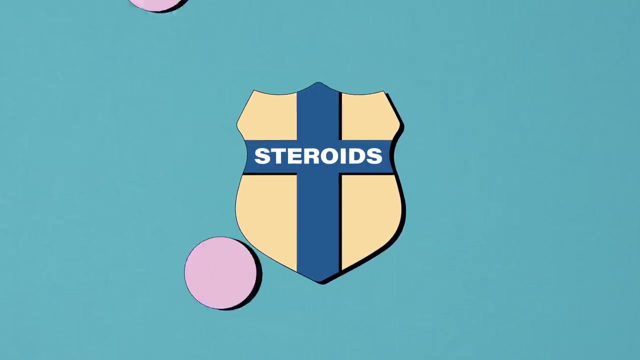 and increased stature and bone mass. Recreational steroid users are more likely to use steroids after the anabolic growth-promoting effects To make muscles grow. steroids first promote protein synthesis. Proteins are essential building blocks of all cells, tissues and organs, including muscles. Steroids also block cortisol, a signaling molecule that drives the 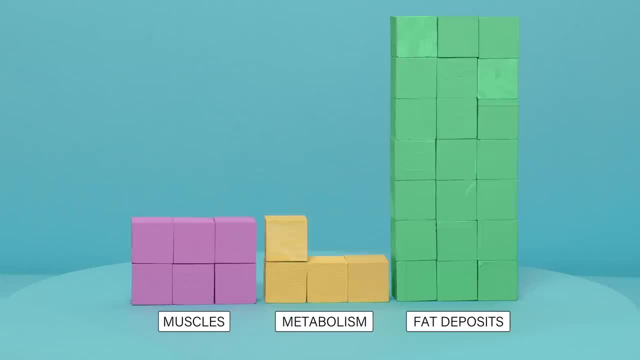 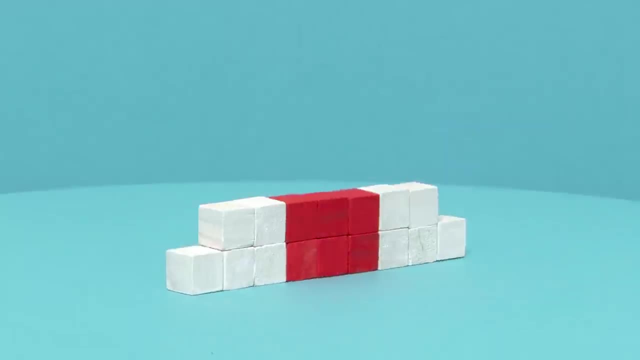 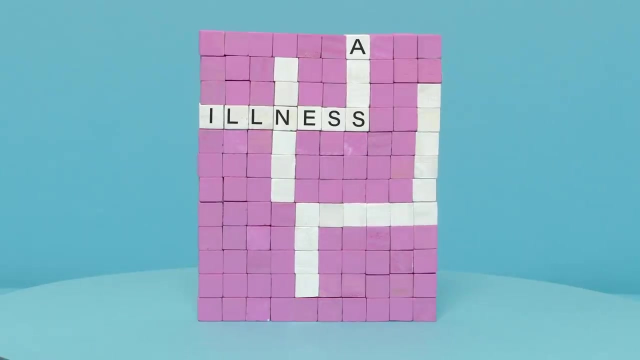 breakdown of substances, including proteins. Finally, they may push the development of muscle rather than fat and boost our metabolism, shrinking fat deposits. These properties make steroids valuable for treating many illnesses and injuries. They can help people with wasting illnesses like AIDS and certain cancers, maintain muscle mass and help burn. 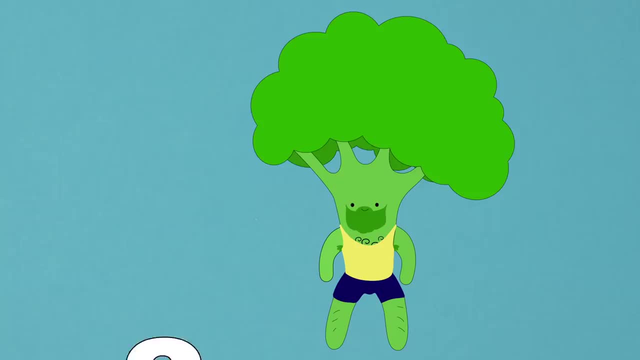 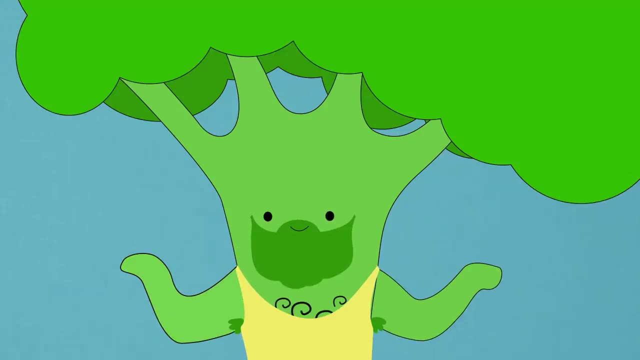 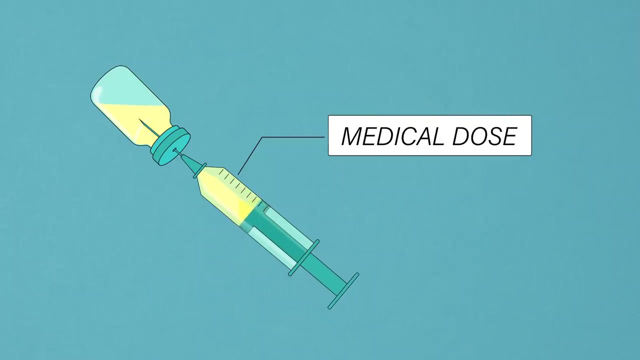 victims recover lost muscle tissue. So if steroids are used as medicine, they must be safe to use recreationally, right? Well, it's not that simple. To create the desired muscle growth, recreational steroid users must typically take doses, orders and use steroids to improve muscle mass, muscle mass and bone mass. In addition, recreational steroid users are more likely to use steroids after the anabolic growth effects, such as muscle mass, muscle mass and bone mass, than those prescribed for a medical condition. Long-term, high-dose steroid usage can have both undesirable and outright harmful effects. some of them dependent on factors like age, sex and underlying health conditions. We're not sure what all the risk factors are, but we do know recreational steroid use can cause problems to mature before they're done growing, causing growth defects. Adolescents are also most at risk for the harmful psychiatric effects of steroid use.